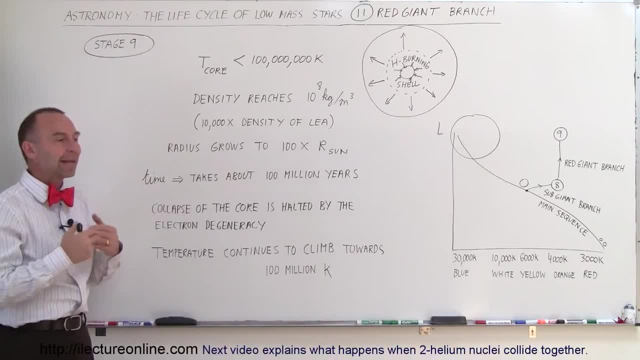 closer or any into a more denser environment and the electrons push back to the point where that became balanced, and that's what we call the electron degeneracy. The electron degeneracy is those electric, electric repulsive force between the electrons that halted any further collapse of the core. At that point the core would have reached the density of 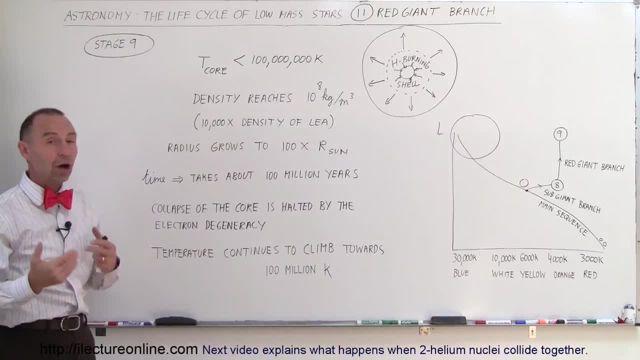 10 to the 8 kilograms per cubic meter. 10 to the 8, that's 100 million. 100 million kilograms or 200 million pounds per cubic meter. That is about 10 000 times the density of- and I forgot letter there. 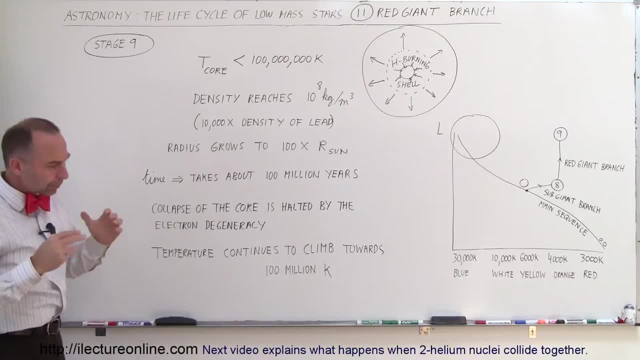 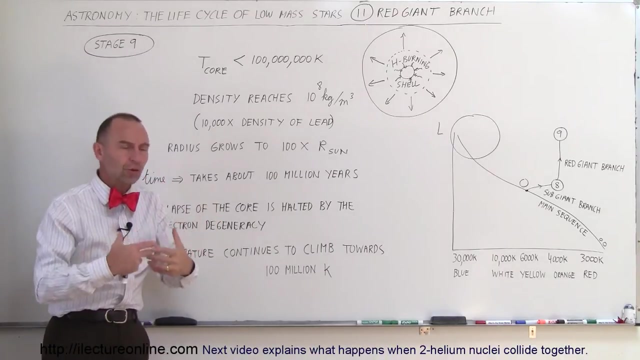 of lead. So core is extremely dense. the the the collapse of the core has been halted by electron degeneracy. core temperature is still below 100 million kelvin, because at 100 million kelvin helium will begin to fuse. so the core is not yet fusing helium, but what is happening is that around 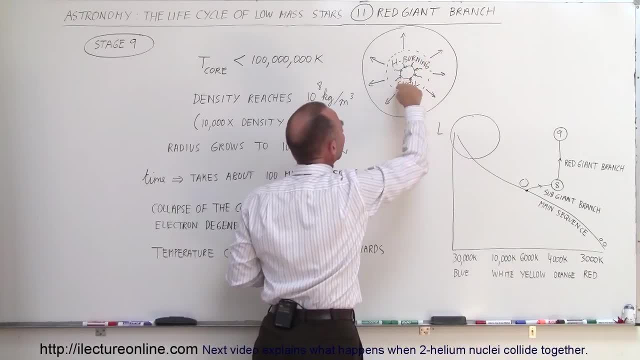 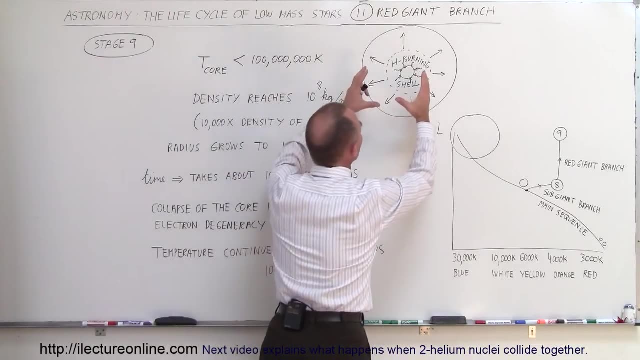 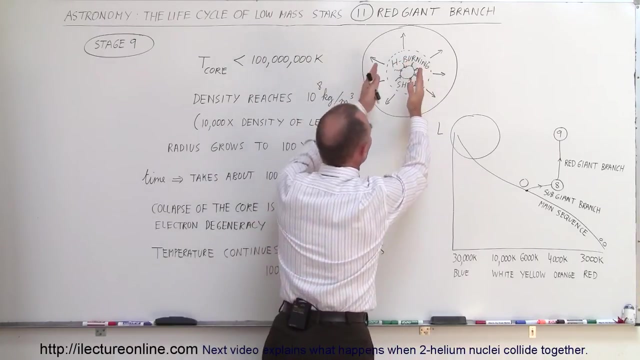 the, the core, this region right here, which we call the heal, the hydrogen burning shell. it is just ferociously burning hydrogen into helium, causing the star to continue to expand. so, even though the core had collapsed, a very dense, dense region down here at the center of the star, the rest of the 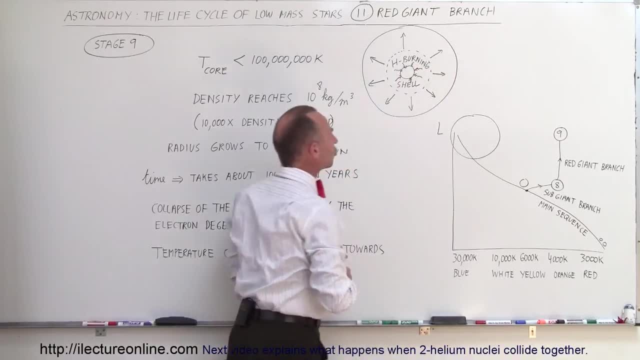 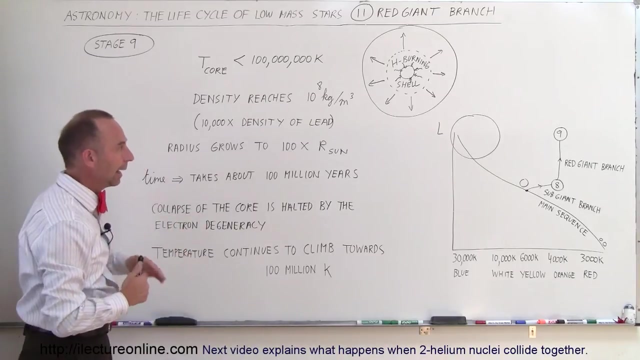 star continues to expand by all this ferocious hydrogen burning into helium, and the star just grows and grows and grows in size. in addition to that, radiation is also pointing towards the core and the core continues to heat up because of the fusion process that's happening around the core. 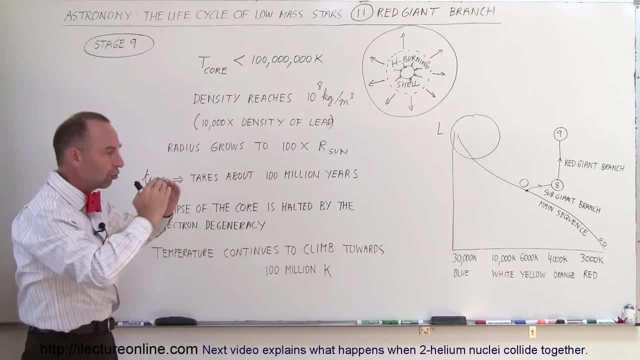 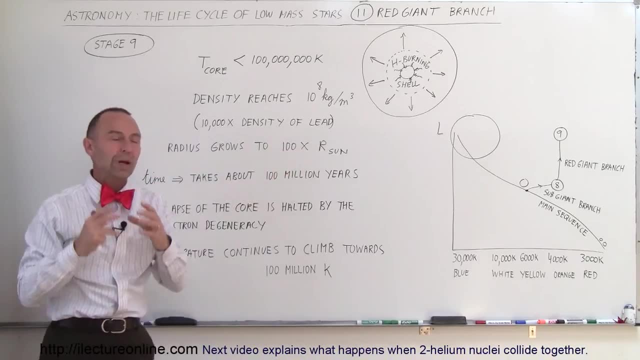 and temperatures keep going up. the collapse has halted the star continues to grow, and continues to grow and continues to grow until the radius of the star is now 100 times the original radius. Imagine the sun with a radius about 700 000 kilometers- at present about 400 000 miles, growing to about a hundred. 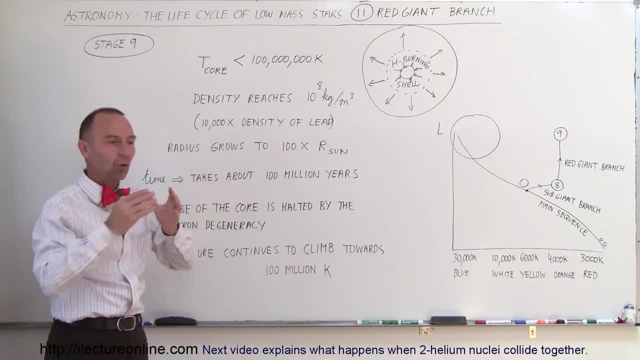 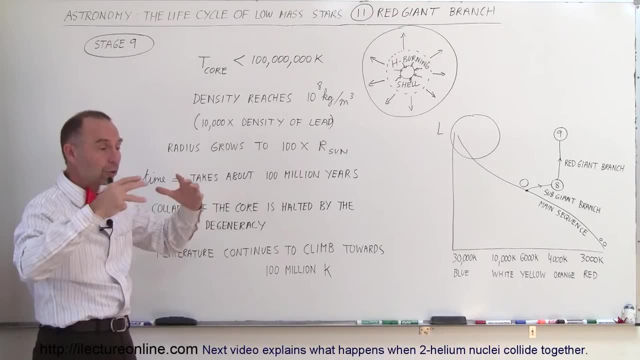 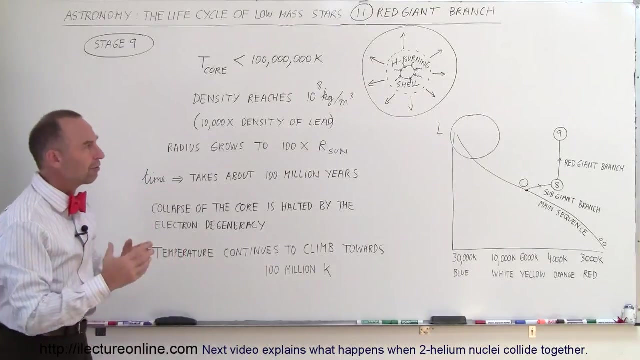 times that radius, 40 million mile radius, or 80 million miles in diameter. imagine a star of that size. well, our sun will eventually do that. it will continue to grow, continue to grow, and that is called the red giant branch. it is now truly turning into a red giant, driven by 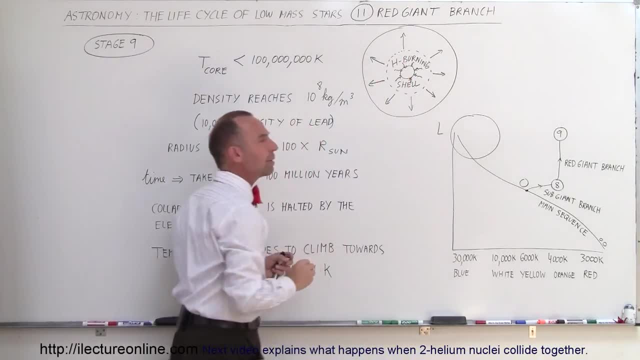 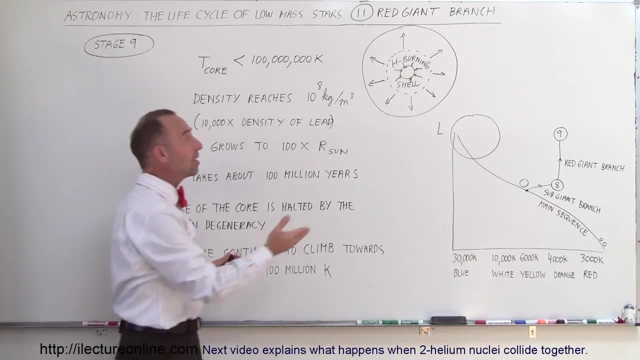 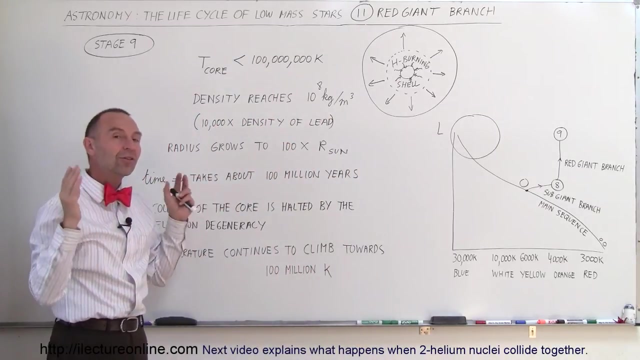 the helium burning of the shell around the core, tremendous temperatures being formed, being being generated and just continuing to push the star against gravity to enormous size. now, since the the edge of the star is so far away from from where all the fusion process is taking place, the star on the surface is relatively cool, probably about 4 000 kelvin. 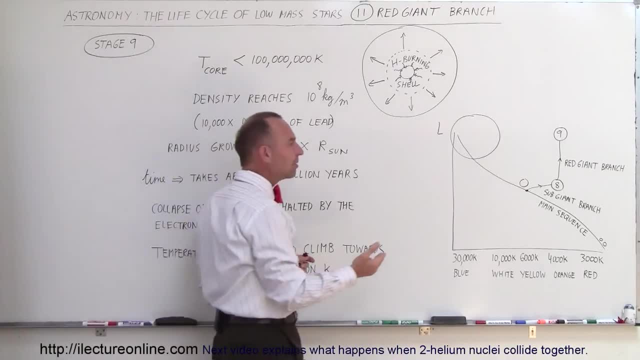 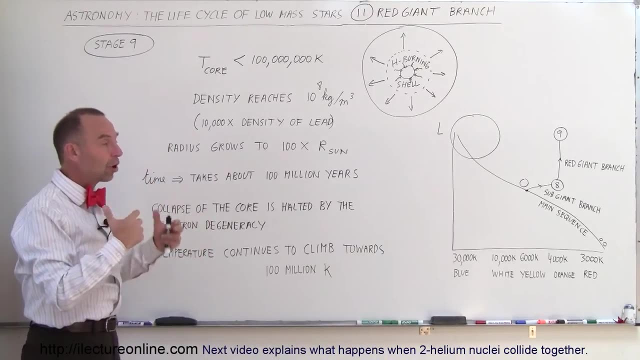 now, how long does that process take? it's estimated that process takes about a hundred million years. we can come up with that estimate based upon looking at these stars as we as we draw on the hr diagram from these big clusters. the big clusters gives us a really good sense of how. long these various processes take by the number of stars that you can find in each stage from a cluster. so, yes, we know that it takes about 100 million years for a star to go from the main sequence all the way up to becoming a red giant, but it's not yet truly a red giant in the sense. that in the core the nuclear fusion process hasn't restarted to the next stage yet. so the collapse is of energy from the sun and the Moon is halted by the electronன, halted by electron degeneracy, and the temperature continues to climb towards 100 million Kelvin. 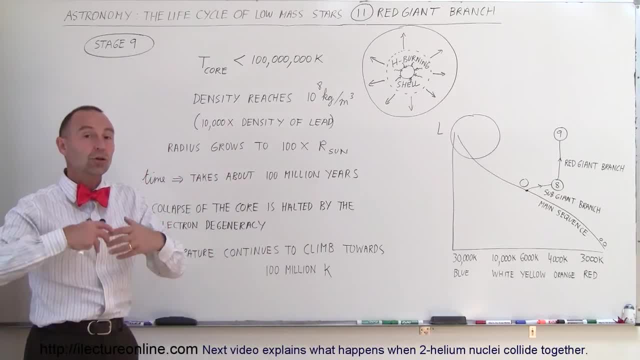 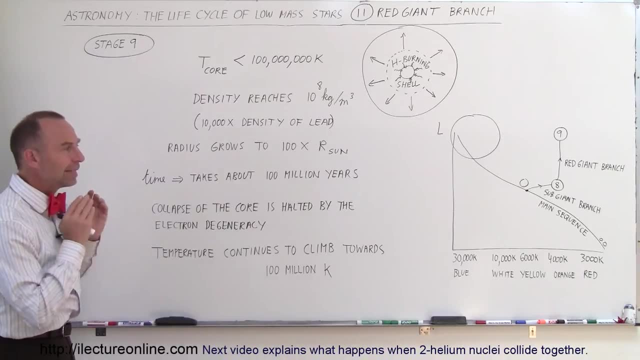 At 100 million Kelvin the star becomes a different star. Now the nuclear fusion process will re-engage in the core, burning helium into carbon. But that hasn't happened yet. That is yet to come, when the next stage happens. So now we're in stage 9 of the star, where 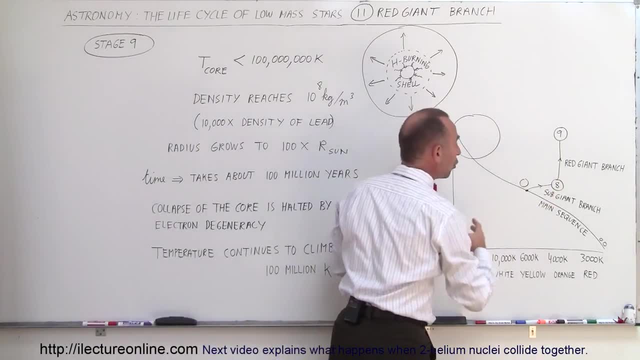 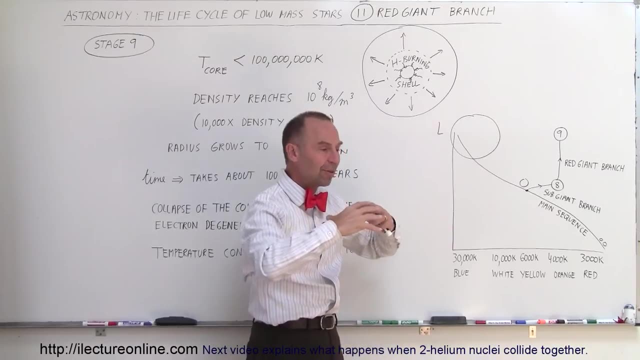 we're creeping up on the red giant branch. Notice the luminosity of the star is increasing by tremendous amounts, not because the edge of the star is getting warmer, but simply because the size of the star grows tremendously. We know, by the amount of the climb on the 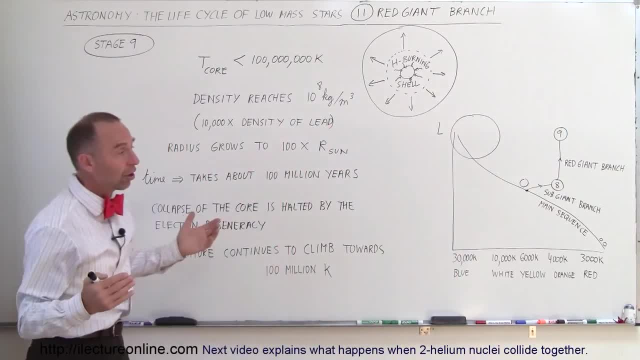 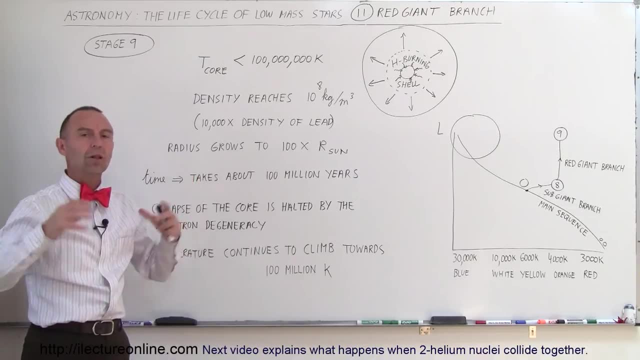 red giant branch. how much bigger the star has to get. Now imagine a star that is so big that currently Mercury and Venus would probably be swallowed by the Sun. When the Sun grows to be that big, it will grow beyond the orbit of Mercury and beyond the orbit. of Venus, and Earth will become the closest planet to the Sun. What will happen to Mercury and Venus? Well, as the Sun continues to grow and the orbit continues to expand, and finally the orbit gets to where Mercury is, Mercury will simply be vaporized. It will be swallowed up by the Sun and, vaporized, become part of the Sun. 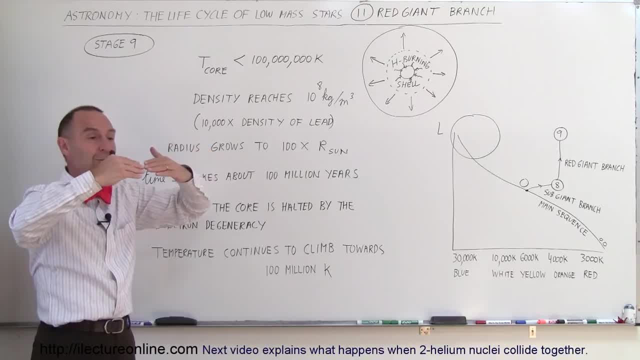 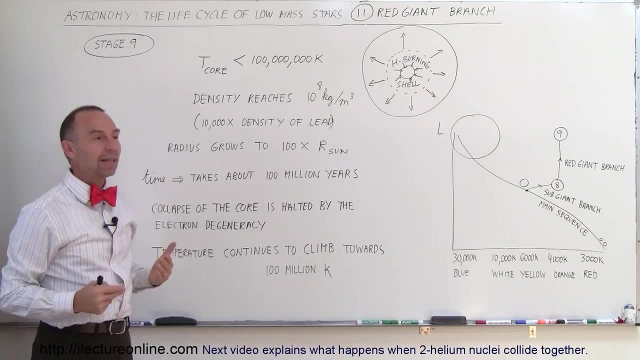 And the Sun will continue to grow until it reaches the orbit of Venus. and if it reaches to the orbit of Venus, Venus will be vaporized and it will disappear and become part of the Sun And that will probably stop. And then, if you were able to stand on the surface of 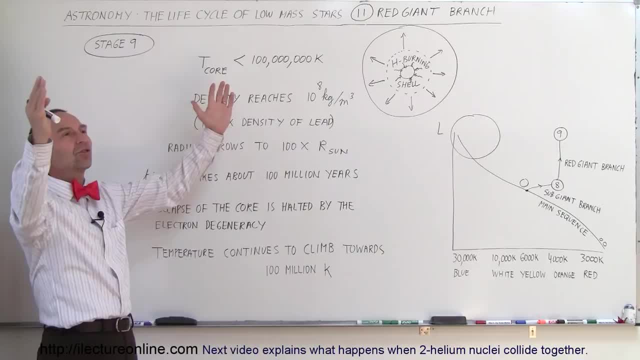 the Earth looking up at the Sun. 5,, 4,, 3,, 2,, 1, go. 5 billion years from now, a quarter of the sky would be taken up by the Sun. It would be huge in size, of course, At that point, the temperatures on the Earth, the surface.